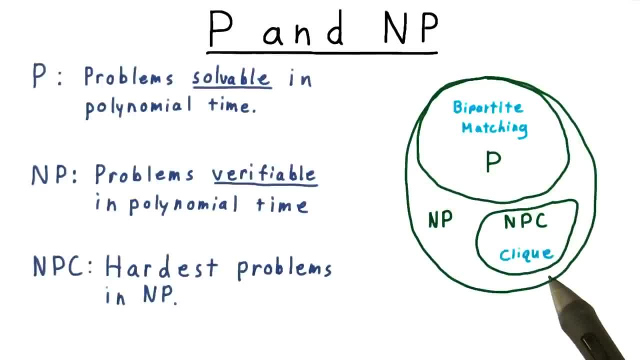 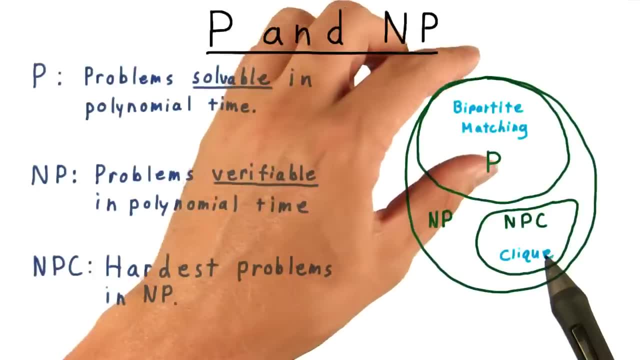 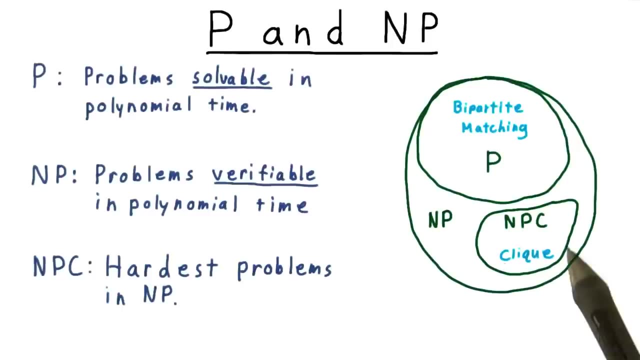 we can efficiently transform into an NP complete problem. Therefore, if someone were to come up with a polynomial algorithm for even one NP complete problem, then P would expand out in this diagram, making P and NP into the same class. Finding a polynomial solution for clique would do this. 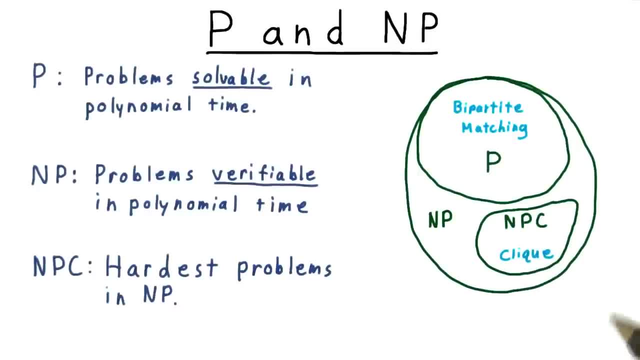 So we say that clique is NP complete. Since solving problems doesn't seem to be as easy as checking answers to problems, we're pretty sure that NP complete problems can't be solved in polynomial time And therefore that P does not equal NP. 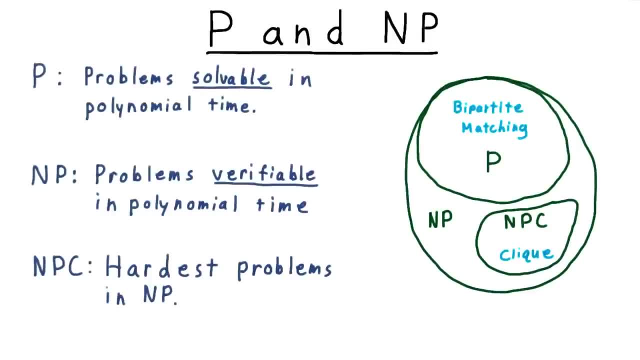 To computer science novices, the difference between matching and clique might not seem to be a big deal, And it's surprising that one is so much harder than the other. In fact, the difference between a polynomial solvable algorithm and an NP complete one can be very subtle. 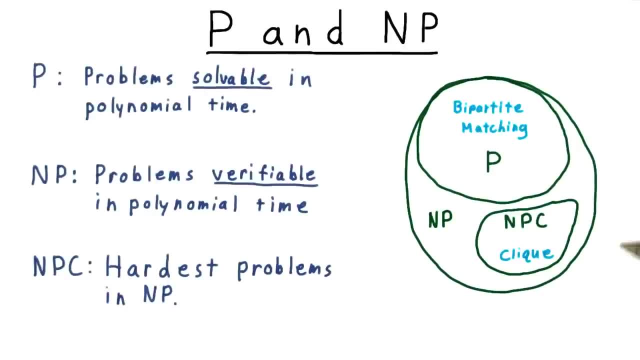 Being able to tell the difference is an important skill for anyone who will be designing algorithms for the real world. 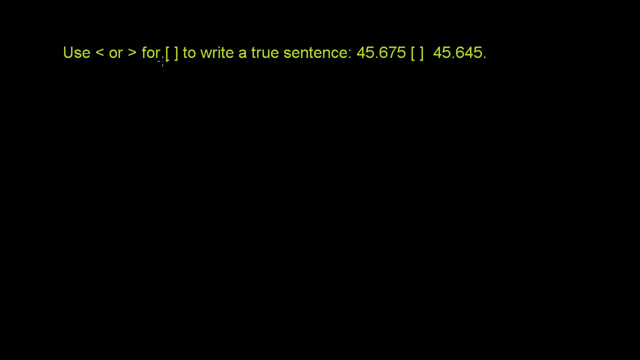 Use less than or greater than for this little brackets thing to write a true sentence. So they essentially want us to say whether 45 and 675 thousandths is greater than or less than 45 and 645 thousandths. So let's look at each of these numbers. I'm just going to write them on top of each other. 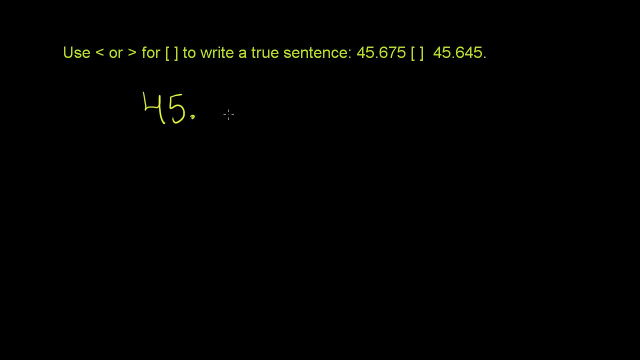 So the first number is 45 and 675 thousandths and the second number is 45 and 645 thousandths. Now, when you look at everything here, the only place where these two numbers are different is in the hundredths place. We have seven hundredths here and we have four hundredths here. 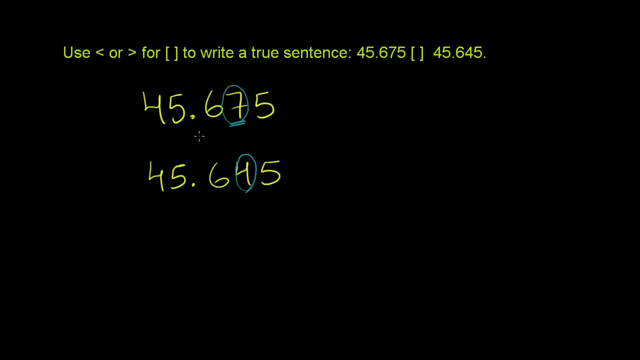 Everything is the same, So this number is going to be greater. This number is greater than 45.645 or 645 thousandths. Let me write that down just to make sure we know what we're doing. 45 and 675 thousandths or 45.675 is definitely greater than 45.645 or 45 and 645 thousandths.